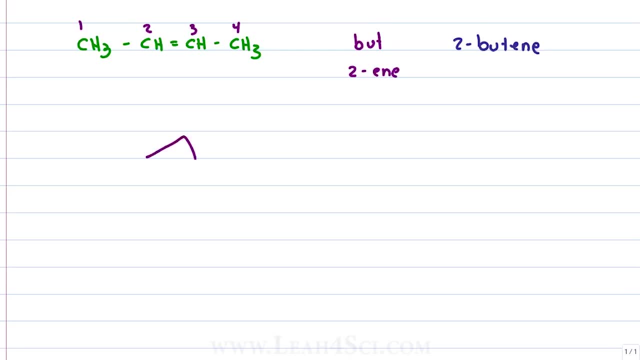 in line structure. I have the option of drawing 2-butene this way or this way, which is correct? The answer is that both are 2-butene, but the first one is the trans isomer and the second is the cis isomer. You've already learned that isomer comes from iso, meaning that it's 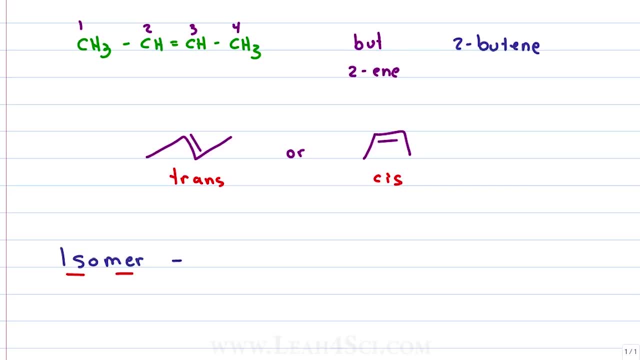 the same and mer meaning units. This is when 2 molecules have the same molecular formula but they're connected differently. Specifically, we're looking at the geometric stereoisomers, where geometric tells us that there's something different in the geometry between the 2 molecules. 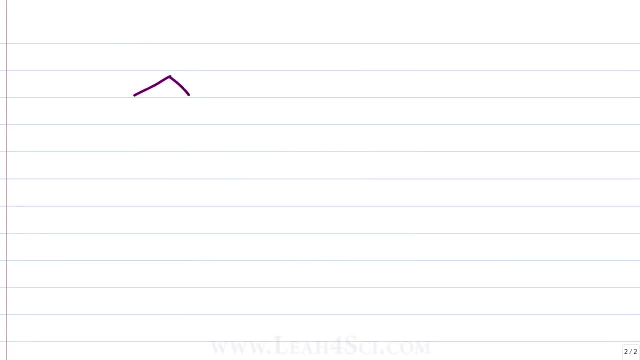 we're comparing. If we try this with the molecule butane, which is an alkane- all single bonds- then we can rotate the bond between carbons 2 and 3. so that the molecule, at any point in time, will look like one of the two configurations. 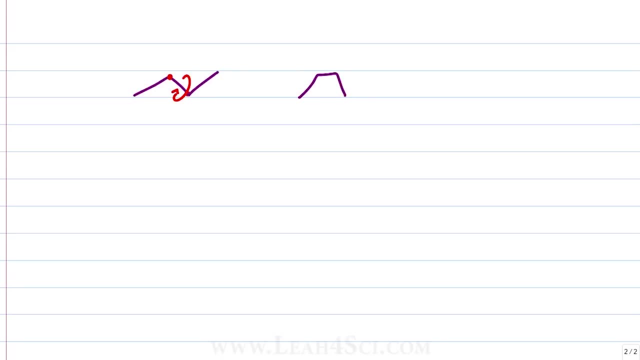 In fact, this is what you study when looking at Newman projections, which is linked below. But to get a geometric isomer, they can't be able to move. you should not be able to turn one into the other and that means they have to be locked in place. 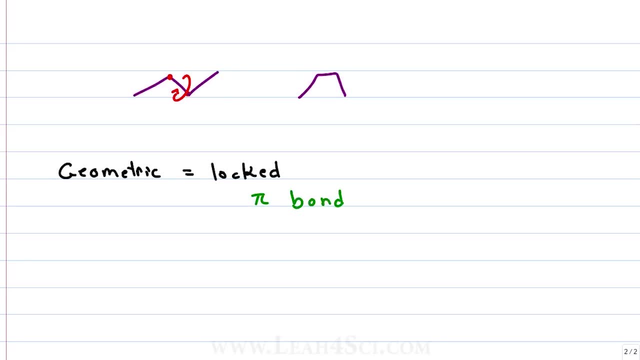 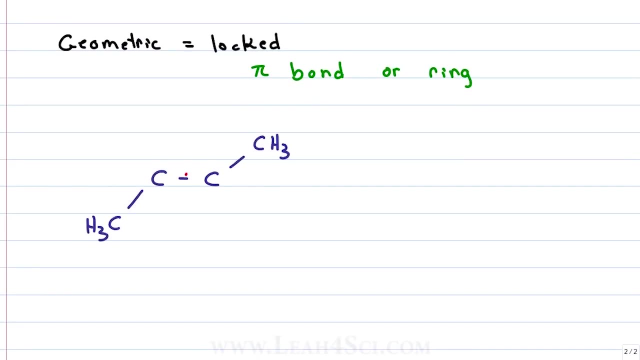 How do you lock the molecule in place? We have two options: a pi bond or a ring. If I look at this molecule with a single bond between carbons 2 and 3, I have free rotation If I add a pi bond between the two carbons. pi bonds, remember, are above and below the 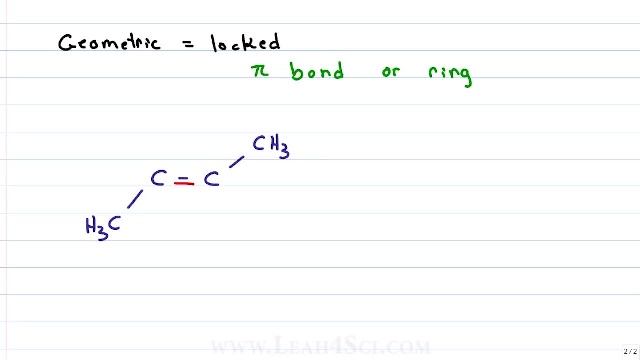 atom. they can't move. the molecule is locked in place and the only way to rotate, to bring this methyl group down, would be to break the pi bond, move the methyl down and then reform the pi bond. Let's take a look at the model kit. 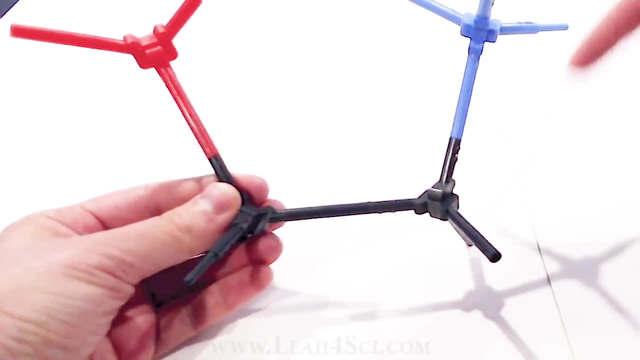 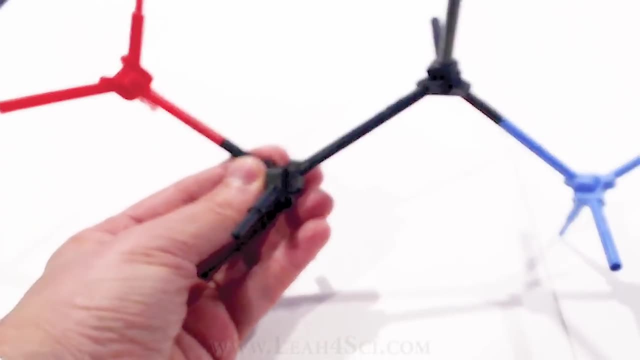 Here we have an alkane with a single bond. Notice that the red and blue substituents are next to each other. but because it's SP3, I can rotate, and now they are opposite of each other, and then I rotate, they are next. 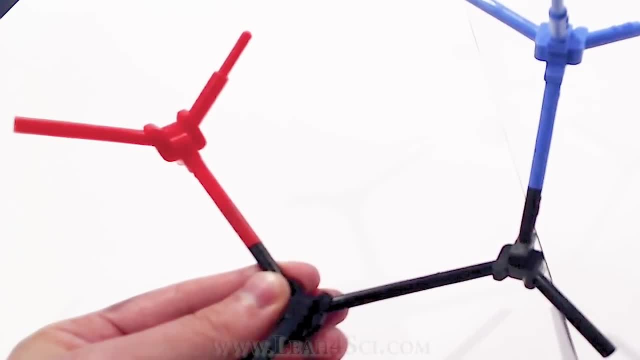 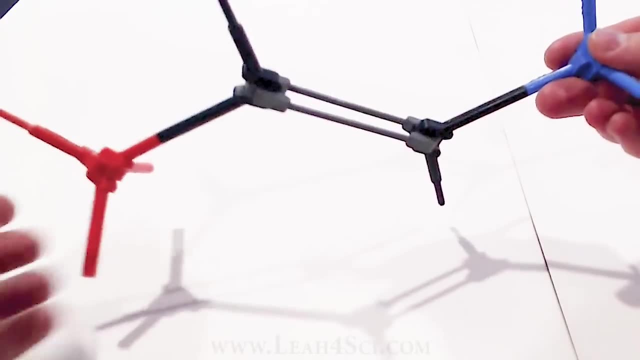 to each other again. The substituents are not locked in place because the carbons are SP3. If I look at a similar molecule, but this time I have two SP2 carbons, pi-bound pulling the substituents. The red and blue substituents are next to each other. 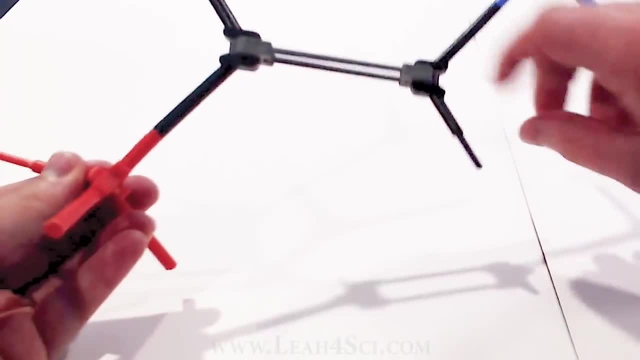 That means if I add one more carbon to one of the other coils I can also get a pi bond now locked in place opposite each other and if I try to rotate I'll break the model kit. It doesn't want to rotate. 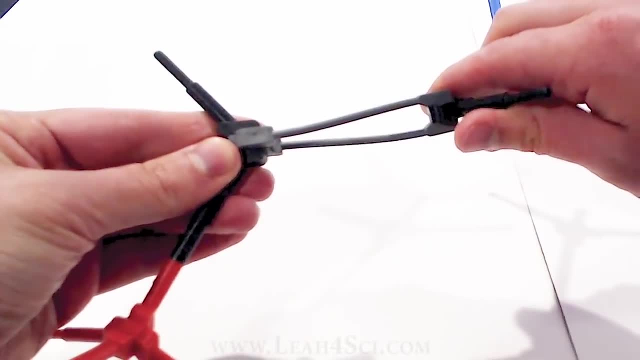 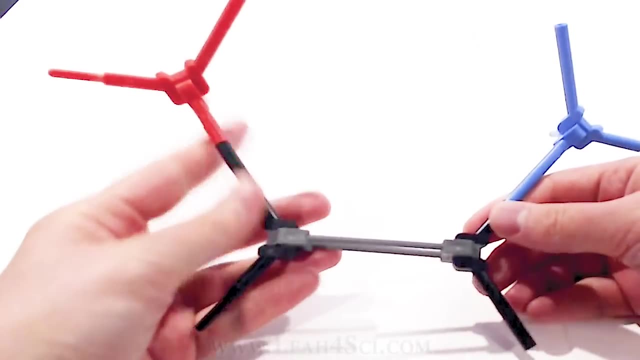 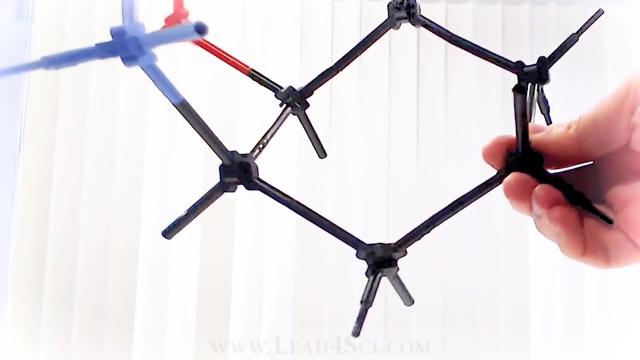 The only thing I can do to get them next to each other is to break the bond and manually move the substituent to the other side and again, now they're locked in place, can't rotate the molecule. We have a similar situation with a cyclohexane where, even though all the carbons in the ring, 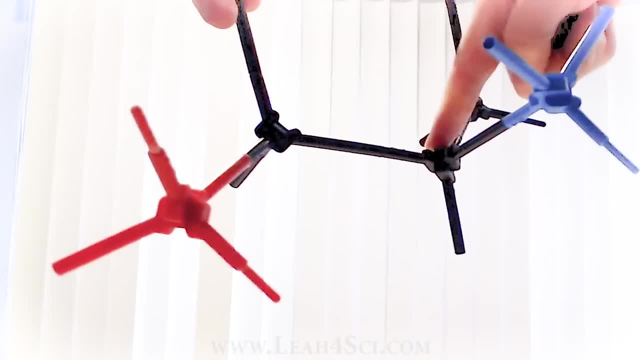 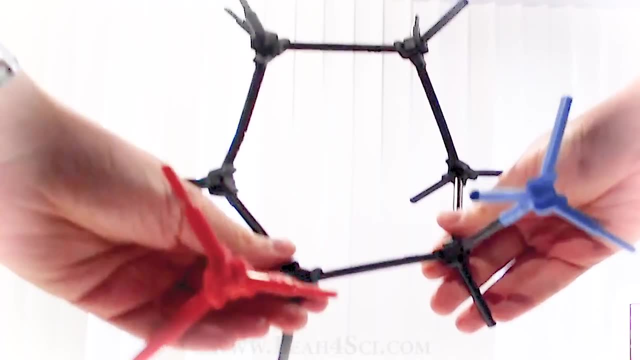 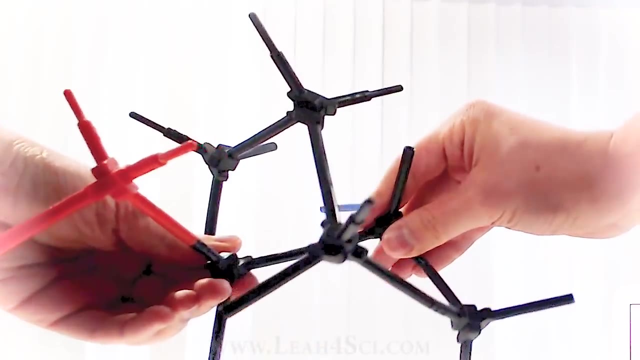 are sp3,. notice that the carbons holding the substituents are sp3, and they can rotate. Watch what happens if I try to move the substituents away from each other. The ring doesn't allow it, The ring is locked in place and this entire thing is going to break if I keep going. which? 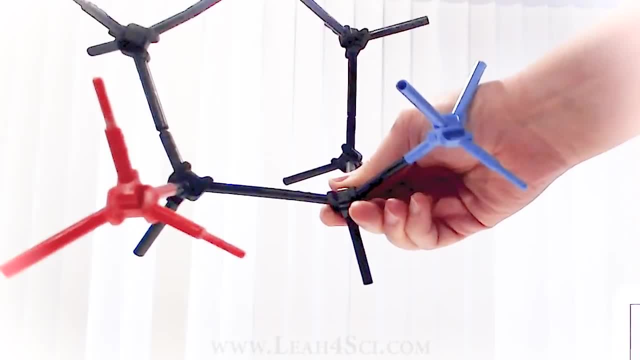 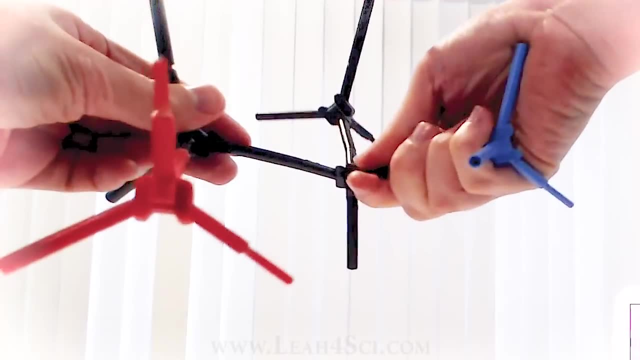 means, even though the substituents are on sp3 carbons in a ring, they're still locked in place And the only way to move them is to rotate. The only way to move them from having two substituents on the same side is to break. 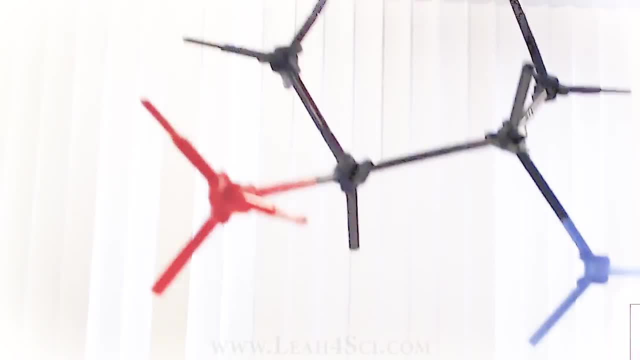 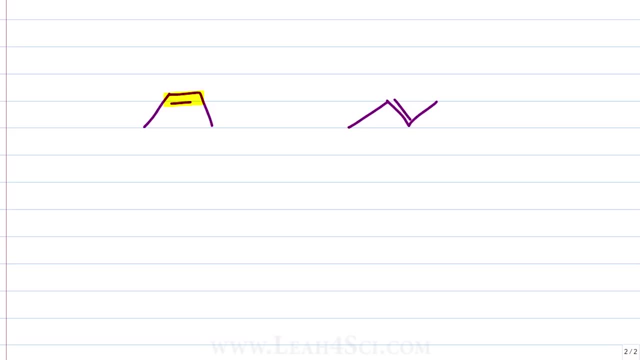 a bond and reform it To identify cis or trans. first identify the pi bond and then look for the substituents that are coming directly out of that pi bond. We don't care about anything else on the molecule except for the very group coming out of the. 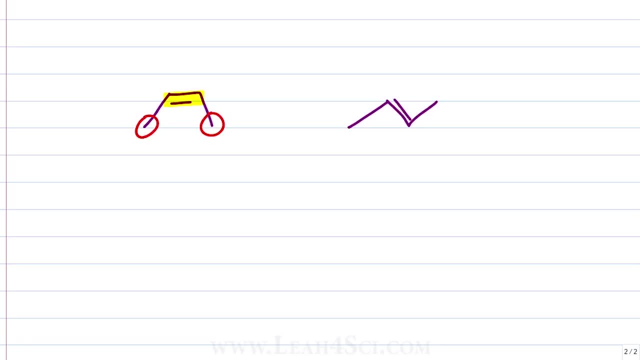 pi bond on one side. compare that to the other side. Once again, identify your pi bond. look at the group coming out on one side and then the other side. How do they relate to each other If they're on the same side? we have the cis configuration, which I like to think of as 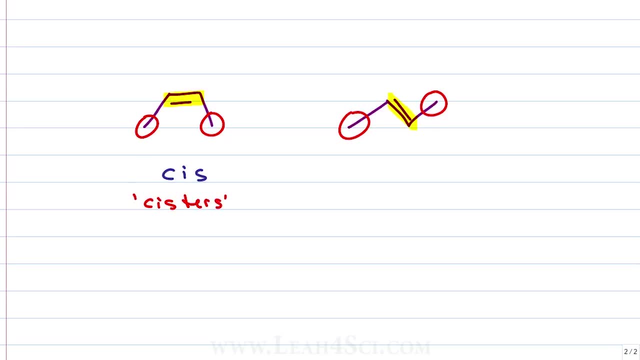 sisters. sisters are together, they're on the same side. If they're on opposite sides of the pi bond, then we have trans. I think of it as transfer away from one side to the other. A note on cis: I drew both of the substituents down. 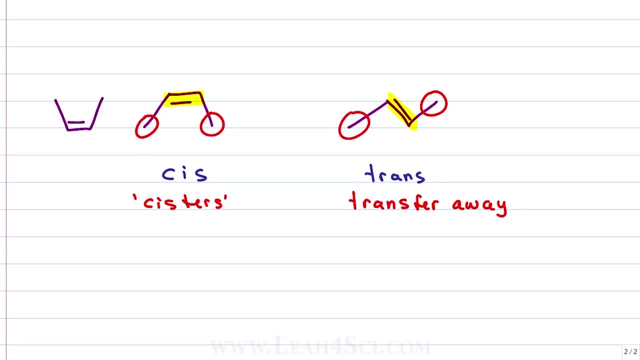 I could just as easily have drawn the molecule this way, with the two substituents pointing up, and it's exactly the same thing, because I can either rotate or flip the molecule and it'll look like this one To name cis and trans alkenes: first learn basic alkene naming from the tutorial link. 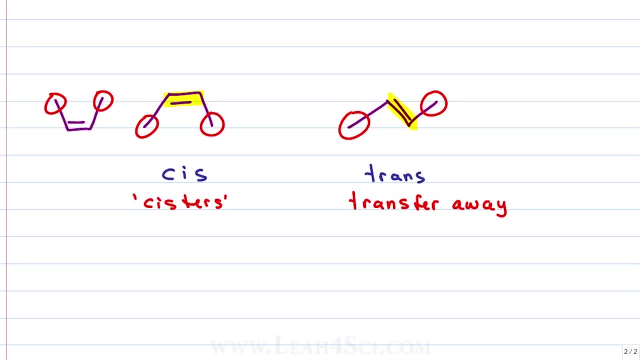 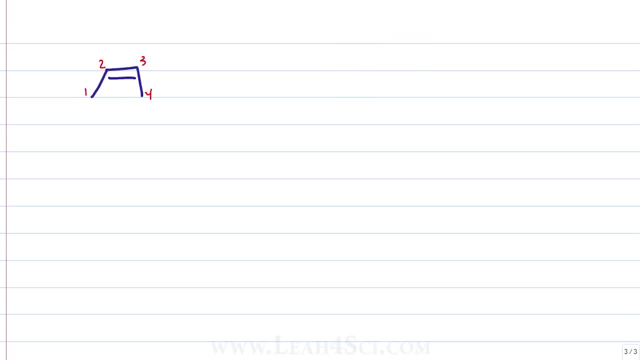 below and then just add cis or trans to the beginning of the molecule. We'll start with our cis molecule. We have cis and trans. We have a total of four carbons, giving me a first name of bute, a pi bond in the molecule. 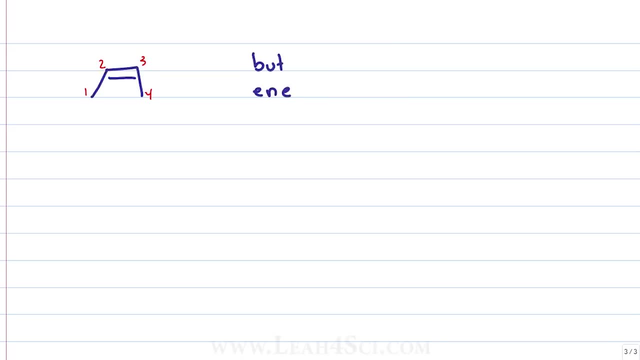 giving me a last name of ene. the pi bond occurs at carbon two. always use the lower number, giving me two ene and the substituents are on the same side. they're sisters. that gives me cis To put the name together. bring cis in front of the name, then drag the two in front of. 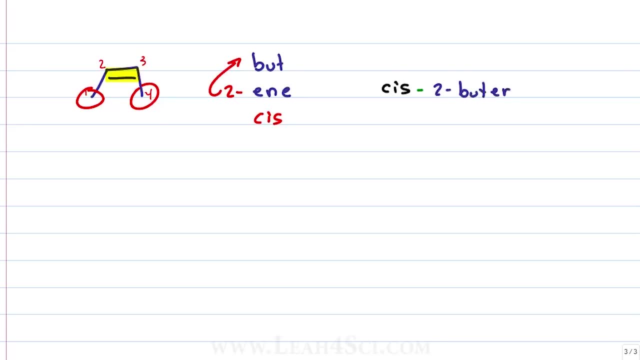 bute giving me cis-2-butene. We're gonna start with our cis molecule. We're gonna start with our cis molecule. We're gonna start with our cis molecule. Now let's try the trans version Once again. we have four carbons in the parent chain. first name of bute: a pi bond starting. 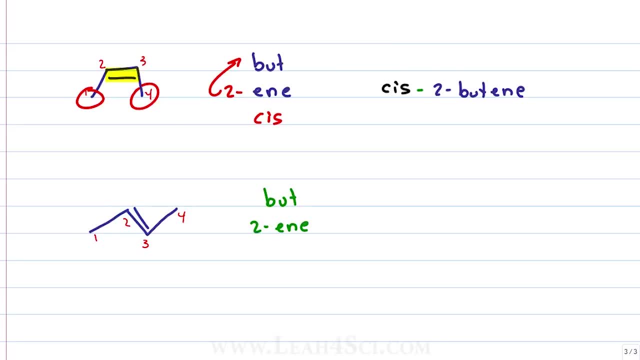 at carbon. two. for a last name of 2-ene. the substituents on the pi bond are facing away from each other or transferred away from each other, giving us trans. Put the name together. we have trans. bring the two in the front butene. 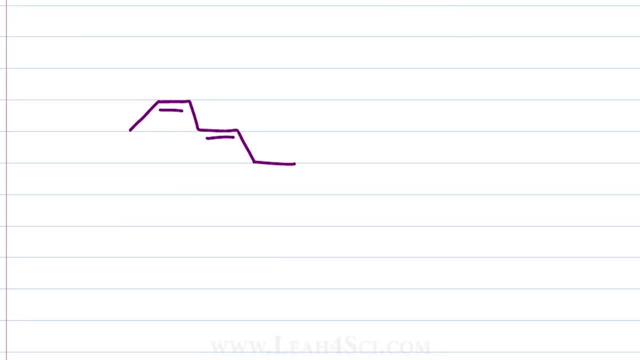 What if we have more than one? What if we have more than one pi bond in the molecule? We start the same way. First we'll number to get the total lowest set of numbers, In this case seven, gives us a first name of hept. 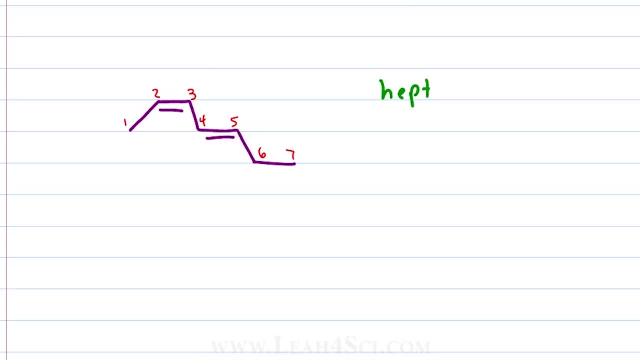 We have not one but two pi bonds, so the last name would be diene di, to specify two and then a number for each one. so we know where they are. First one starts at carbon two. second starts at carbon four, giving me 2,4-diene. 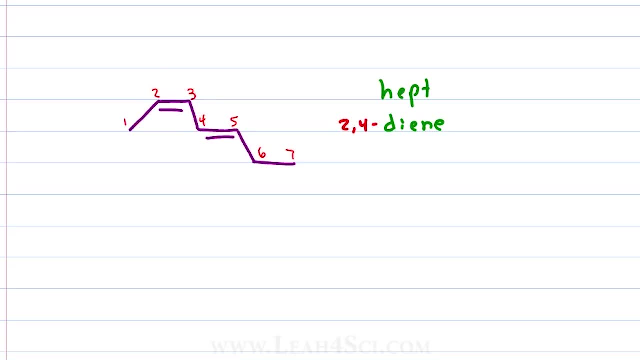 We're gonna start the same way. We're gonna start the same way. We got two butes here: three pi bonds, two pi bonds, two trans, three pi bonds and a three pi bond, One by three-diene. and, last but not least, are they cis- or trans? 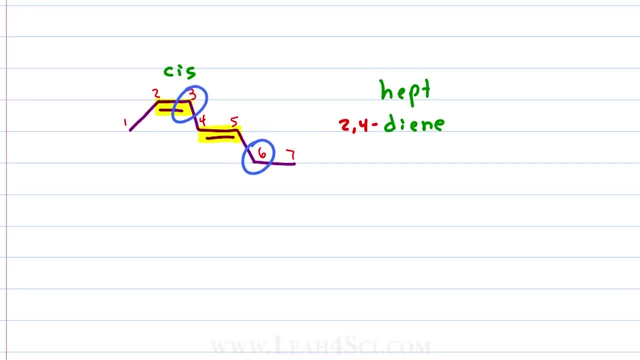 The pi bond starting at two has the substituents facing on the same side. remember we're looking at just the carbon coming out of that pi bond. The pi bonds starting at four has the substituents on opposite sides, giving me trans For this name. we can't simply put cis or trans in the front, because we have to specify. 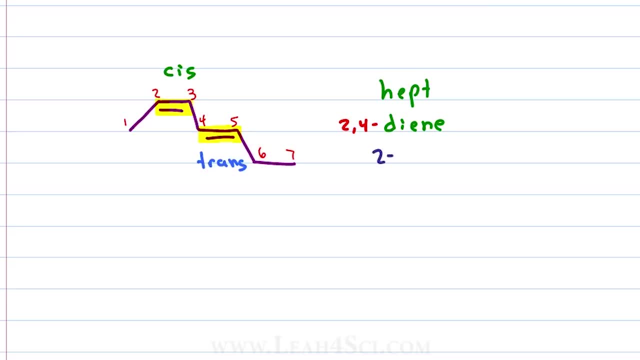 number in front of the designation. that means we need 2 cis and 4 trans at the beginning of the name. Putting this all together, we have the pi bond designations: 2 cis-4 trans. then we bring these numbers out front: 2,4-first and last name, heptadiene for a final name. 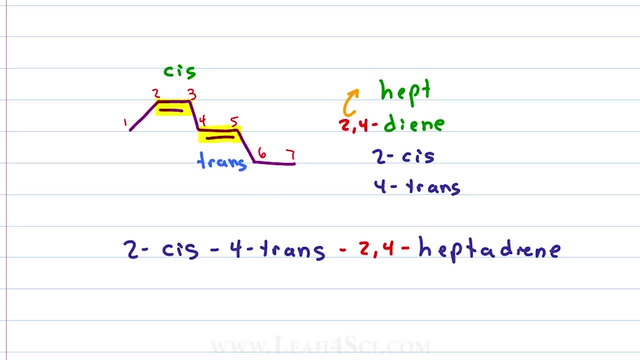 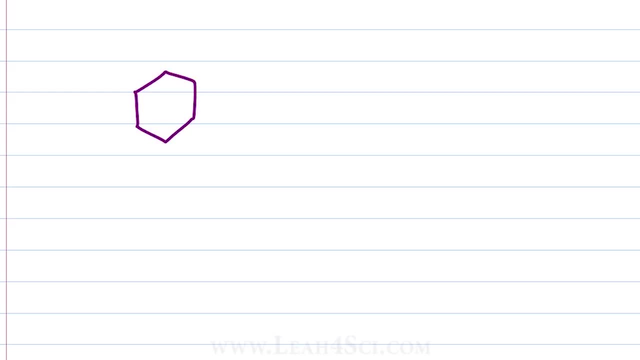 of 2 cis-4 trans-2,4-heptadiene. We said there were 2 ways to lock the geometric isomers in place. The first was a pi bond. second is a ring. With the ring we can have different. 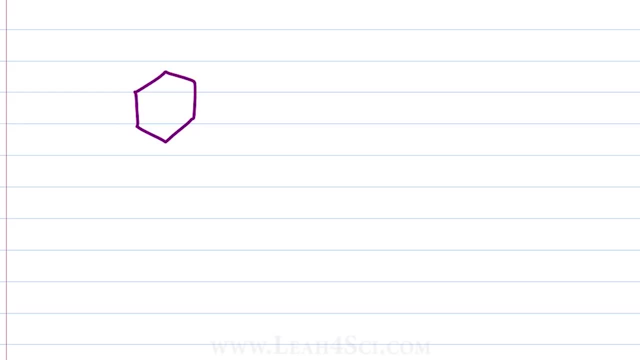 types of substituents, because we're just looking at the relationship. In this case, the substituents on the cyclohexane would be up or down, where you should remember that a wedge tells you the substituent is up and dashes tell you the substituent is down. So we're going to 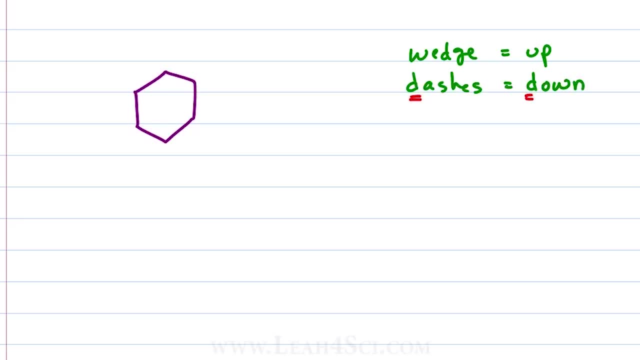 start with the D. If I add 2 methyl groups to this cyclohexane, you'll notice one is a wedge and one is on a dash. They are on opposite sides. they are transferred away from each other. This molecule has the methyl groups trans to each other. That's because 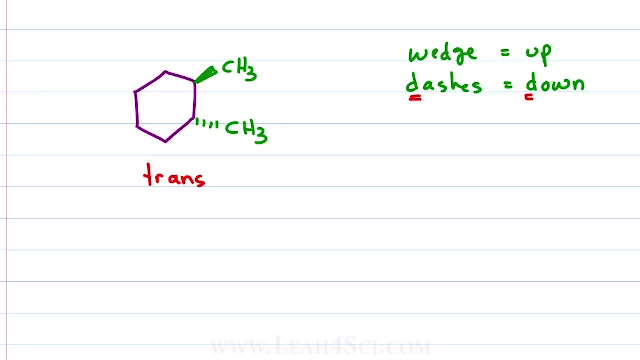 one is up and one is down. It doesn't have to be just methyls. What if I have 2 halogens, Say a chlorine and a bromine? In this case, we're going to have 2 halogens. We're going. 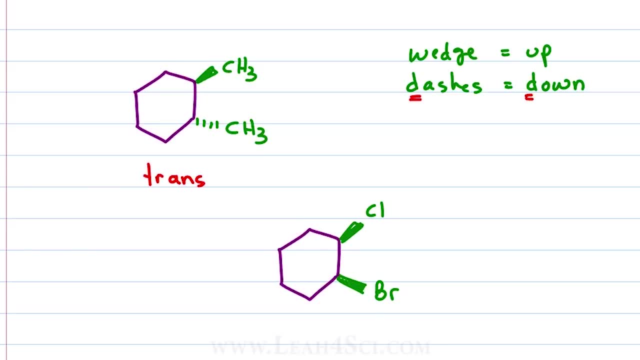 to have 2 halogens. In this case, I can say that the 2 halogens are cis to each other. That's because the chlorine is up and the bromine is up. They're on the same side. they're like sisters together going up making them cis. This is covered in more detail when you 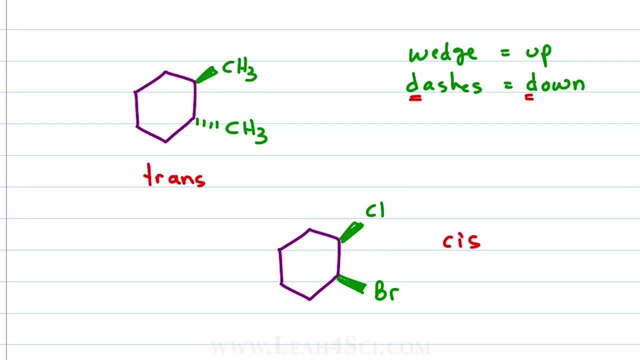 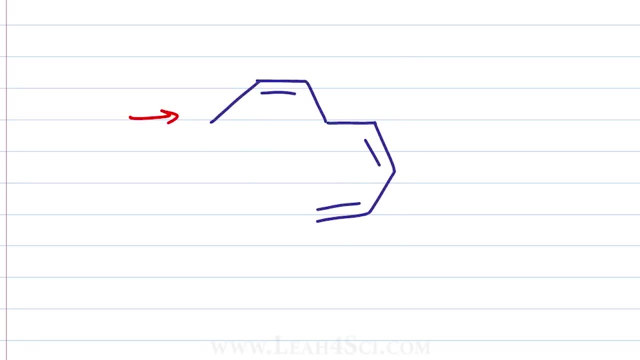